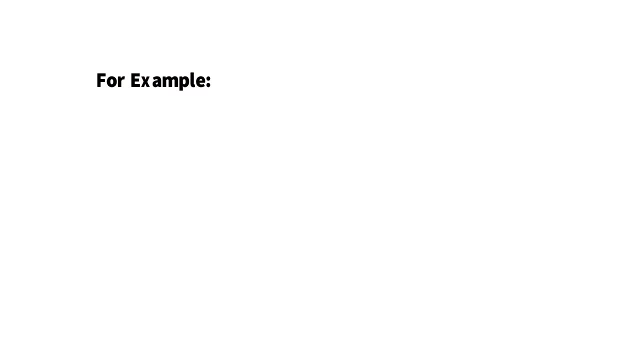 head of a vector. Now, for example, if I have a three vectors- vector one, vector second and vector three. Now, if I have a three vectors- vector one, vector second and vector three. Now, here, if I want to add these vectors, Before adding the vectors, I will join these vectors. 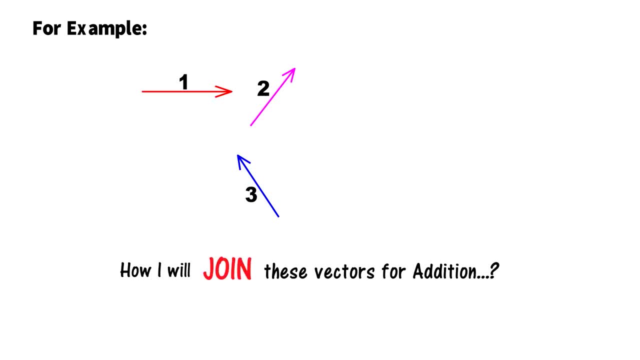 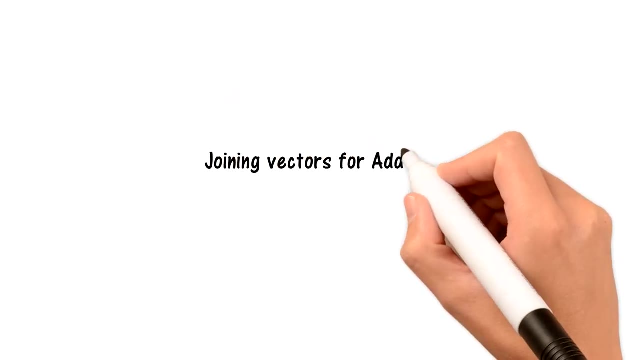 for the addition. Now, how I will join these vectors for the addition. Now to join different vectors for addition, I am going to give you a trick, and remember this trick whenever you are joining vectors for addition. And the trick is very simple, and that is head and tail trick. 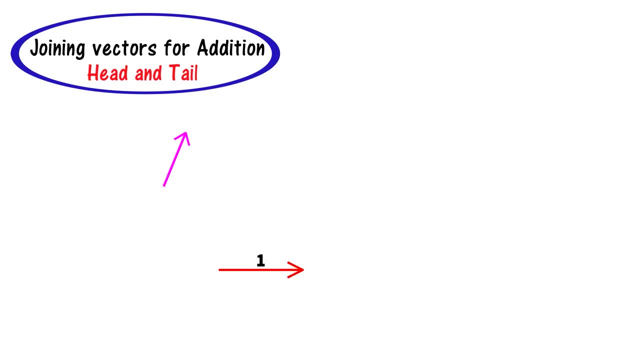 Now what I will do. I will take the first vector Now, I will take the second vector and I will join the tail of the second vector with the head of the first vector, And then another vector. I will take the third vector and I will take the tail of the third vector and I will join the tail. 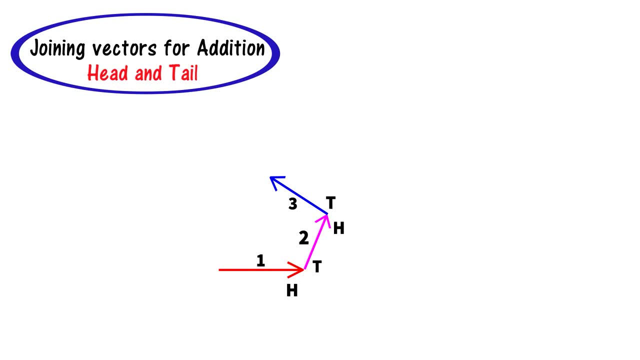 of the third vector with the head of the second vector. So this is the head and tail rule in order to join vectors. for addition, Now how I will add all of these vectors. Then I will use the another trick. The trick is tail and head trick. I will take the. I will join the tail of the first vector. 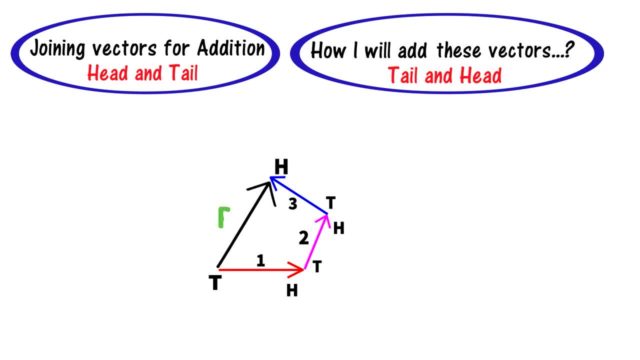 with the head of the third vector, And this is the resultant vector. This resultant vector is actually giving me the addition of these three vectors: 1 plus 2 plus 3.. And remember, resultant vector is a vector which gives the result of all these. 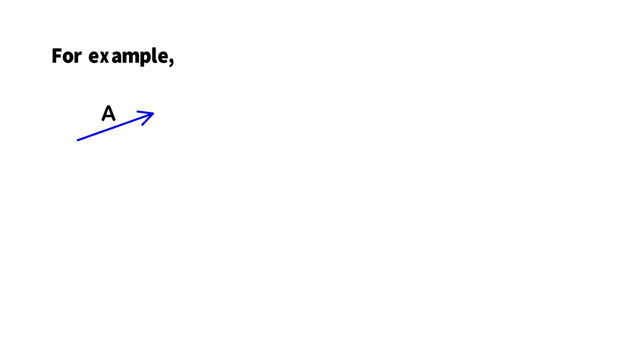 three vectors. Now, for example, if I have two vectors, a and b, and if someone is asking me to find the addition of these two vectors, a plus b- So what I will do? I will take the vectors a and b and I will join the tail of the vectors b with the head of the vector a, And I will then what I 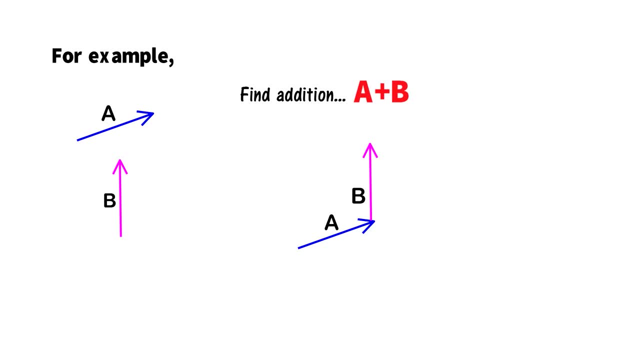 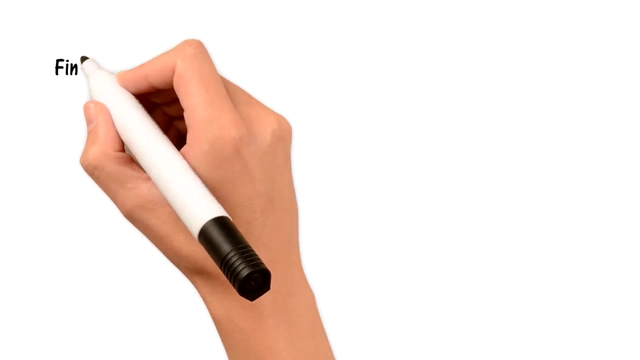 will do. I will take another vector and I will join the tail of the vector a with the head of the vector b, And this is the resultant vector. And this resultant vector is giving me the addition of two vectors: a plus b. Similarly, if someone is asking me now and in this example, to find the sum, 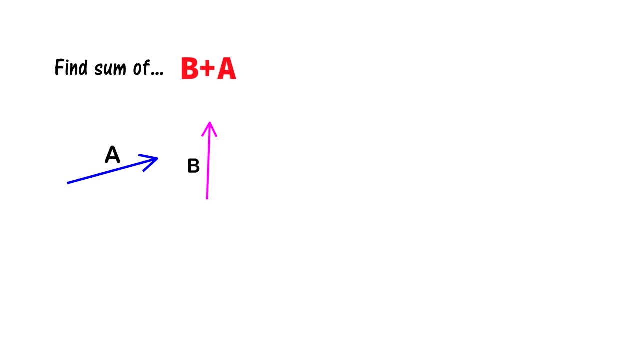 of b plus a vector. So what I will do now, here I am not taking the vector a. Here it is. the question is asking me to find the sum of b vector plus a vector. So I am taking the vector b and then I am. 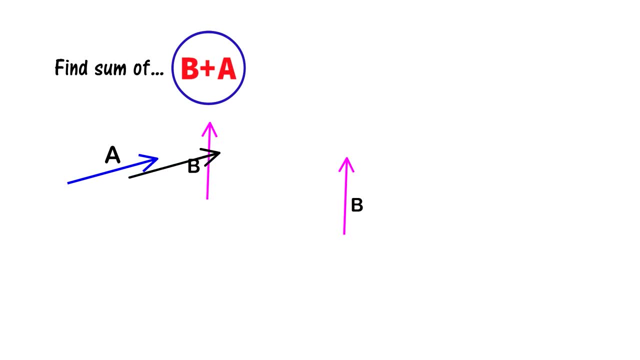 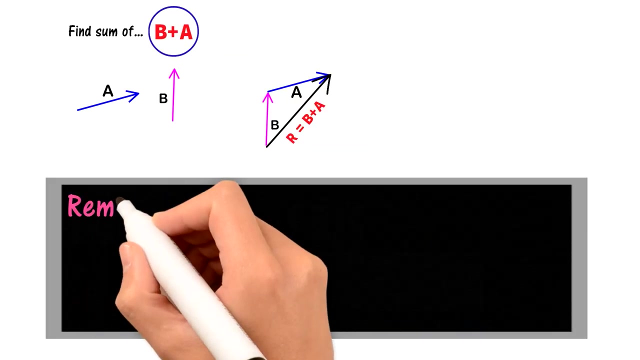 taking the vector a and I am joining the tail of the vector a with the head of the vector b. And now to get the result of b plus a, what I am doing? I am joining the tail of the vector b with the head of the vector a and I am getting b plus a. Remember: a plus b is equal to b plus a. Or we say: 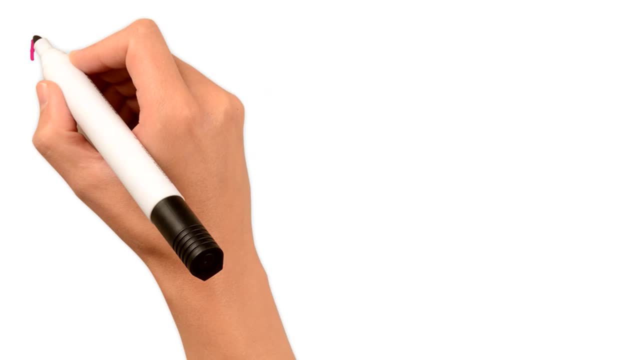 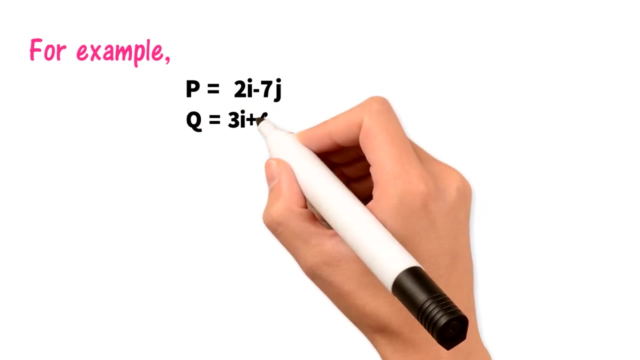 vector addition is commutative. Now, for example, if I have a vector, p is equal to 2 minus 7 and q is equal to 3 plus 4.. If someone is asking me find the addition of these two vectors, p plus q, 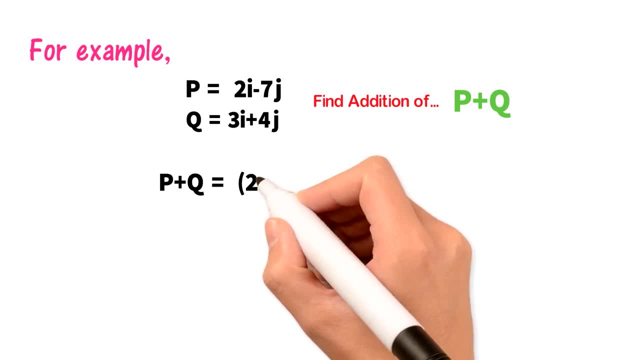 So what I will do? I will take the vector p and I will join the tail of the vector a with the head of the vector a. two minus 7 plus 3 plus 4, and I know 2 minus 7 plus 3 plus 4.. Now here. 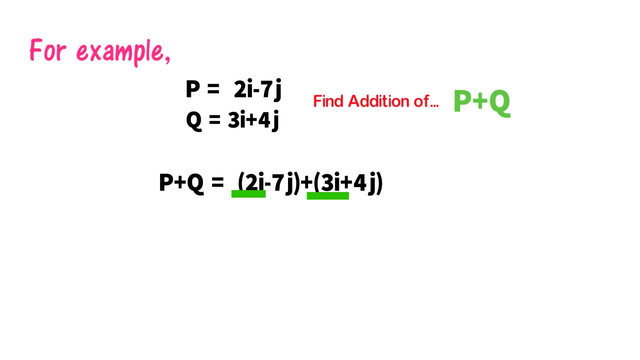 the X part will added with X part and what is is actually a unit vector of X direction and j is the unit vector and the y direction. So X part will be added with the X part and Y part will be added with Y part. So I am getting b plus a- already beside b stuff actually- and k will still. be added with the upper district of the vector. So what I am getting, b plus a and q will be added with a lower district of the vector a. Yes, it is so. Now I haveост Lyman verse. It has well before $1.. 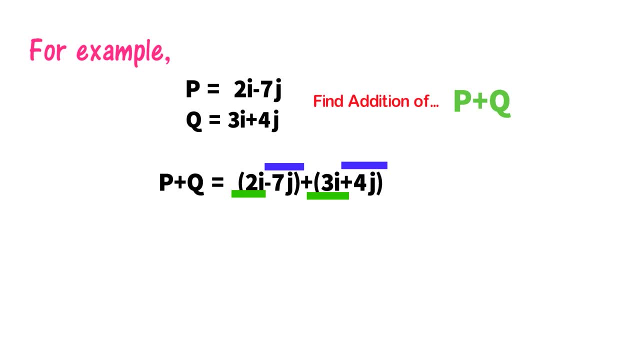 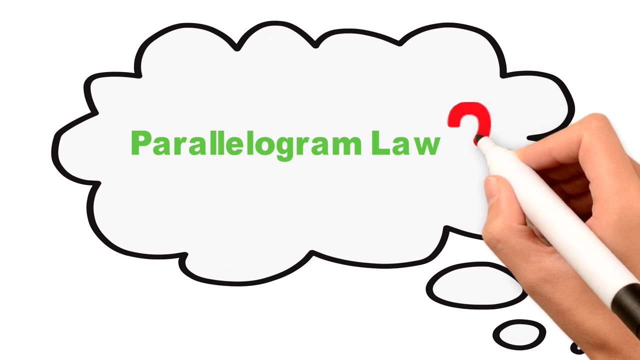 adding X, part 2 plus 3 and I'm getting 5, and its unit vector is I minus 7 plus 4 and I'm getting minus 3 in its unit vector is J. so this is the addition of P plus Q. now, what is parallelogram law? this law was used by Aristotle to 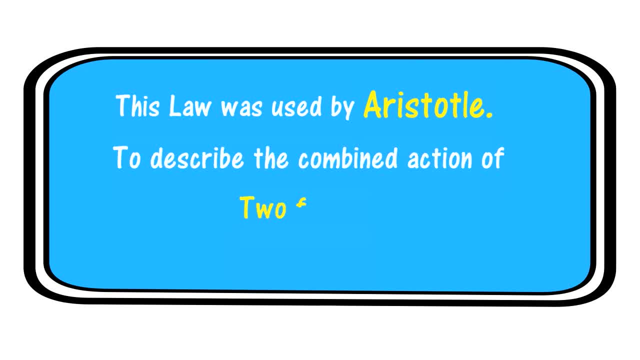 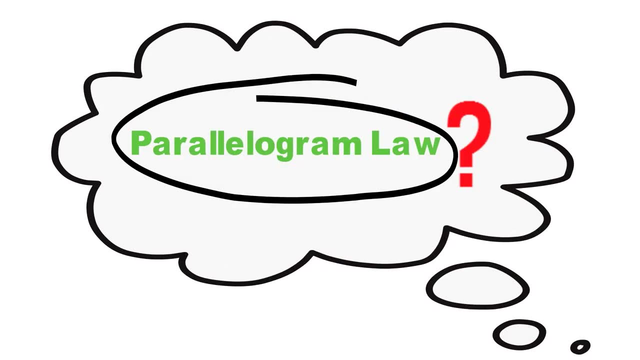 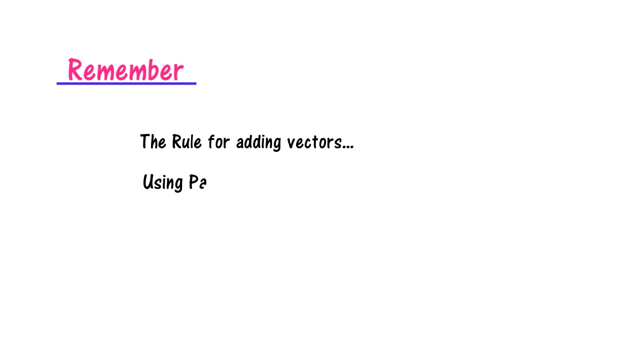 describe the combined action of two forces are two vectors. remember I'm saying two forces are two vectors. we usually use two vectors are two forces in order to add them using the parallelogram law. now, for example, and remember the rules for adding vectors using the parallelogram law, is TNT rule. 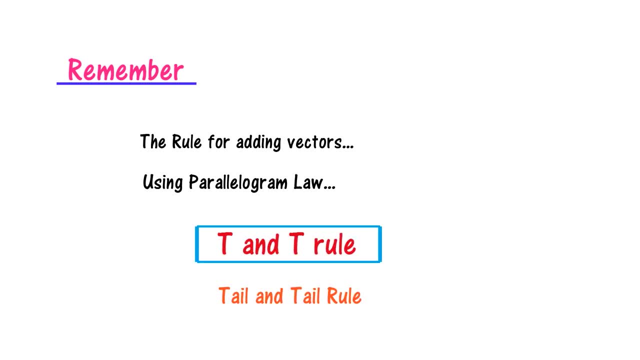 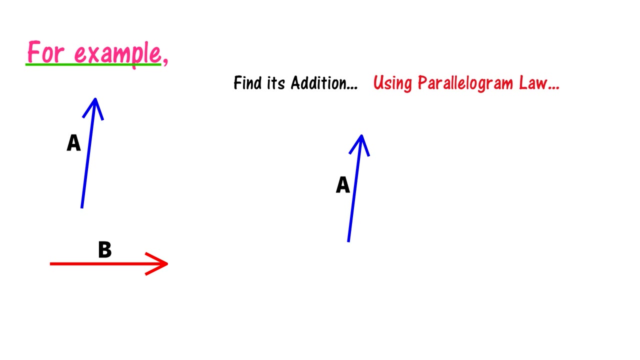 and what is TNT rule? tell and tell rule. so, for example, if I have a two vectors, A and B- and if someone is asking me to find its addition by parallelogram law, so what I will do, I will take vector A- now I am not using the t- Aunt of Victor B to join it with the 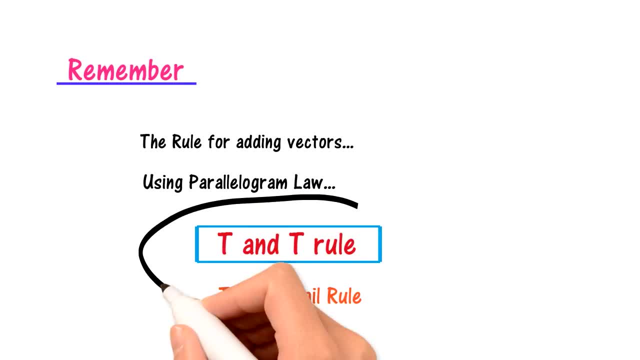 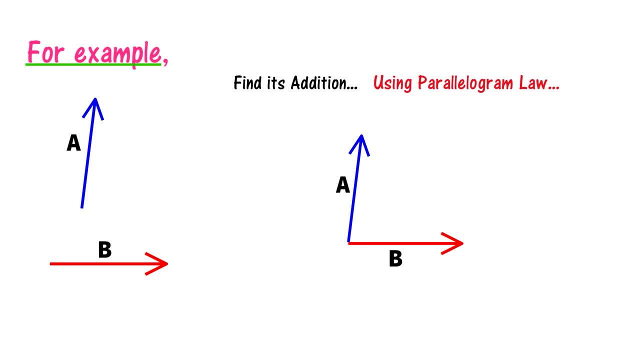 heart of Victor A, not not. I'm not using this thing. I'm using to enter T rules. I am taking with to A and now I am taking vector B and I am joining the Teter Victor be with the Tela Victor, and. and now I'm taking with to B and I am. 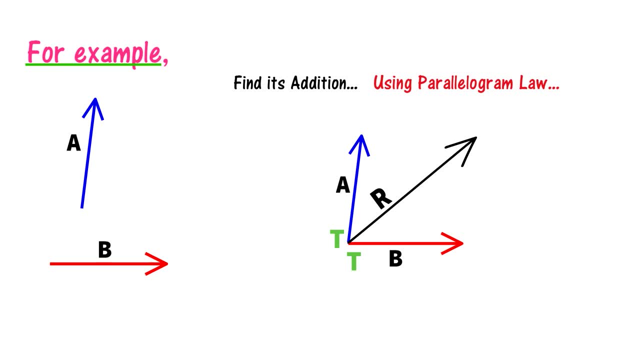 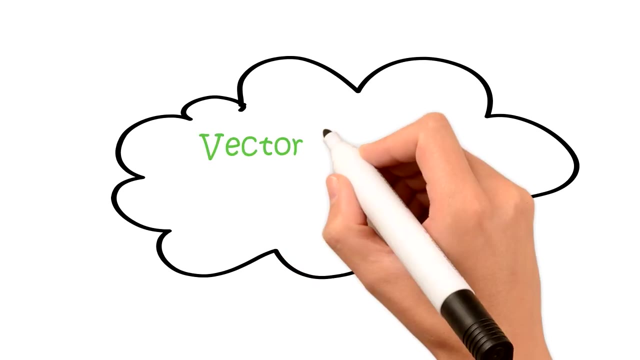 i am taking resultant vector and also keep it in your mind: the tail of resultant vector will be joined with the tail of vector a and vector b and i'm getting this vector resultant vector and it is giving me a plus b. now why vector addition is commutative. for example, if i have: 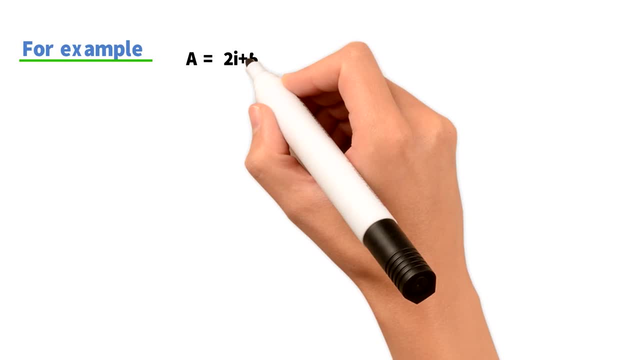 a vector a, which is equal to 2 plus 5, and if i have another vector b, which is equal to 7 minus 2. now, remember, i and j is actually the unit vectors of their respective numbers. now, if someone is asking me to find a plus b, the addition of these two vectors, so what i will do, i will take 2 plus 5.